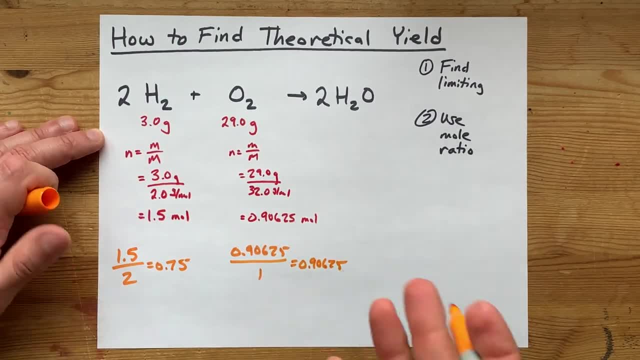 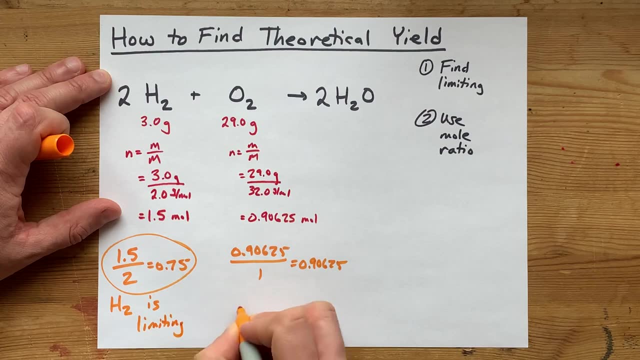 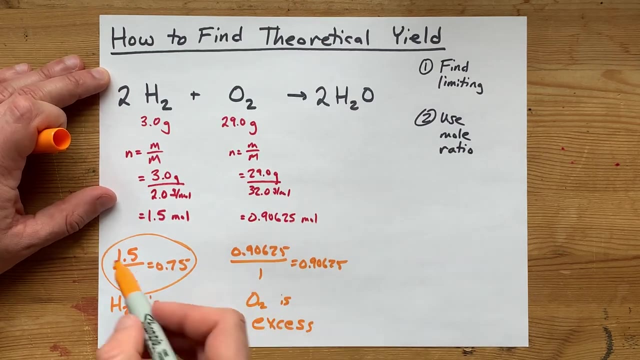 the smaller one corresponds to the actual limiting reactant. Oh, that's this one. So H2 is my limiting reactant here, and O2 is not limiting. The word we have for that is excess. Now, to be honest, I discard these calculations once I've figured that out. 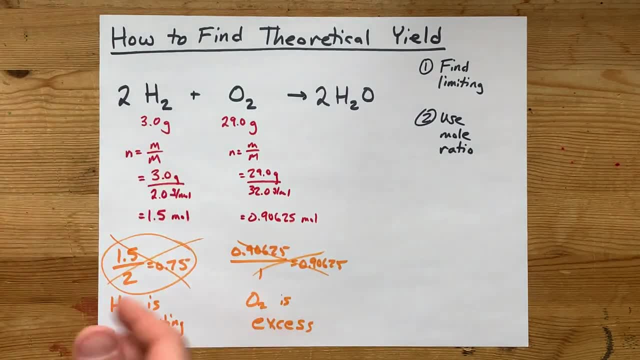 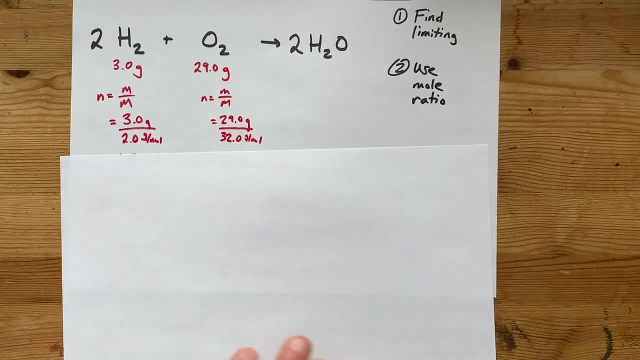 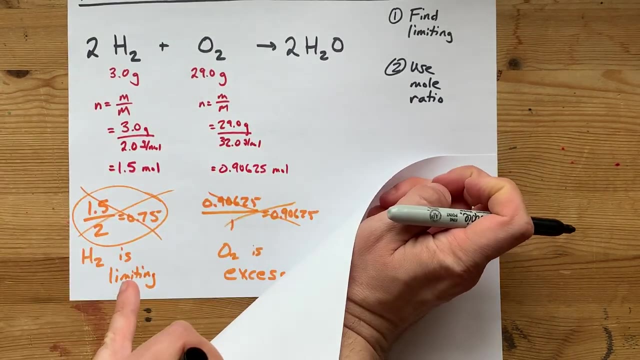 All I needed to know is which one is limiting. Now we're going to use a mole ratio to figure out how much water is made, But the trick is that you have to base that amount off of the limiting reactant, because it's the H2 that's controlling how much water we can even make. It's the limiting. 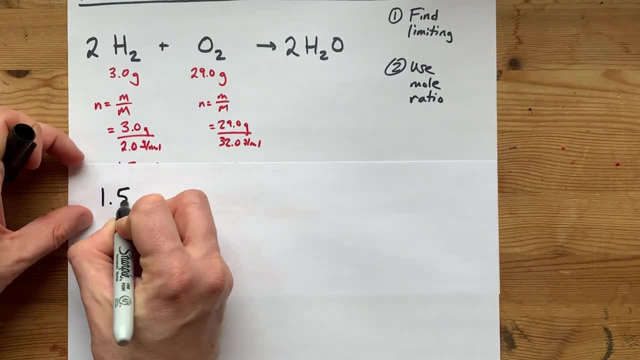 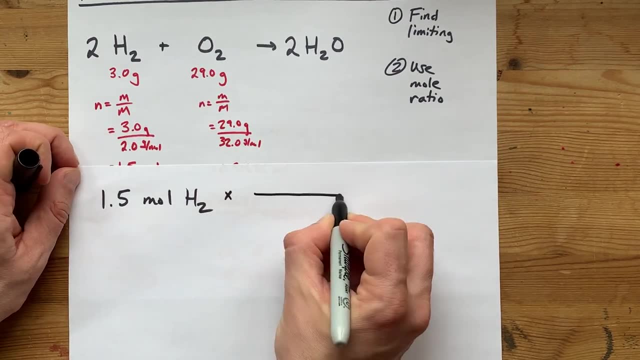 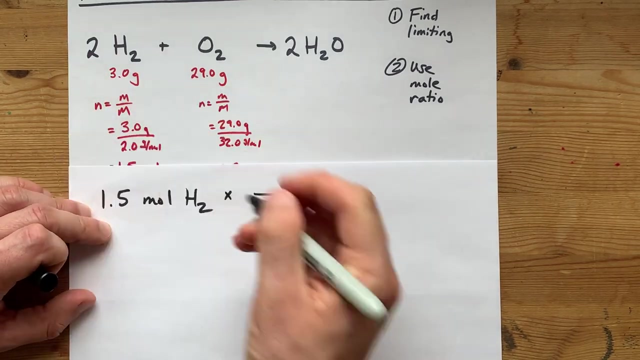 factor. Get it Now. we started with 1.5 moles of hydrogen, See, And we're going to multiply that by a ratio, A ratio On the bottom. I want you to put the coefficient for hydrogen and the fact. 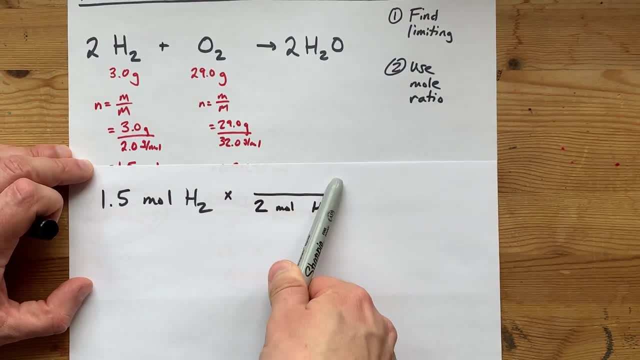 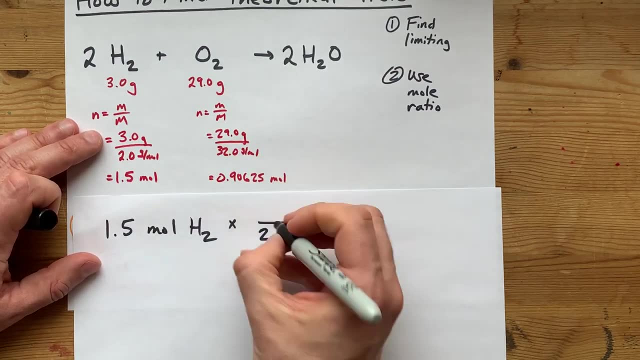 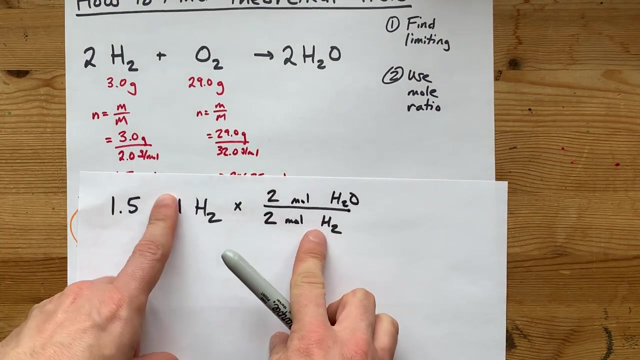 that it is hydrogen. And on the top I want you to put the coefficient of the thing you're trying to find Here, because we're looking for yield, we want to know how much water is made. So we're going to put 2 moles of water in the numerator. The reason, the thing you already know about, goes. 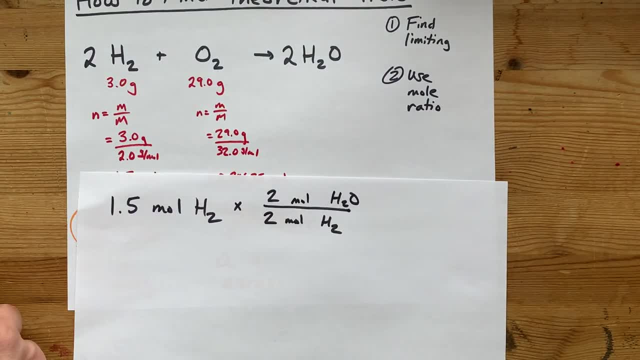 on bottom is so that those units can cancel with each other. Here we have moles of H2 being divided by moles of H2.. Anything divided by itself is 1, and the unit we're left with is moles of H2O. 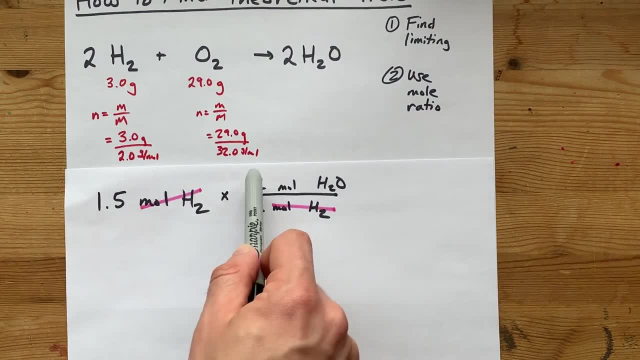 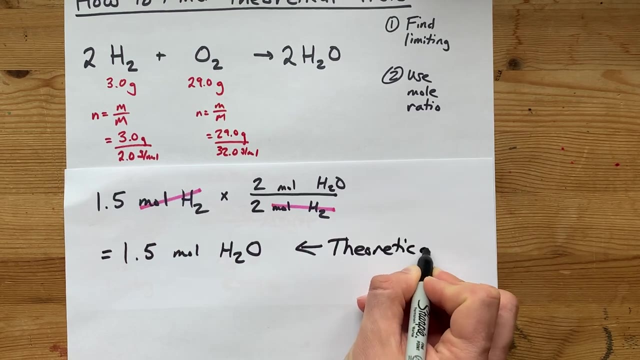 Oh, that's perfect. 1.5 times 2 is 3.. Divided by 2 is 1.5.. 1.5.. So we get 1.5 moles of H2O. That is the theoretical yield. It's as simple as that, It is. 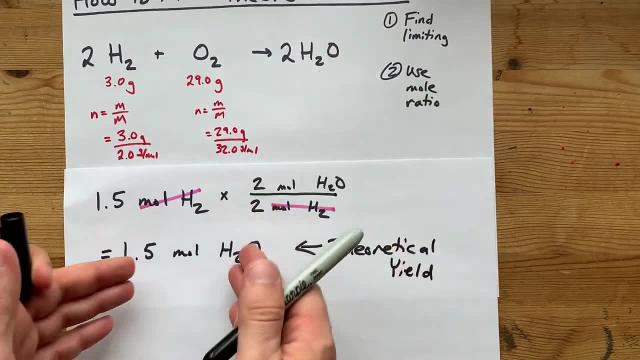 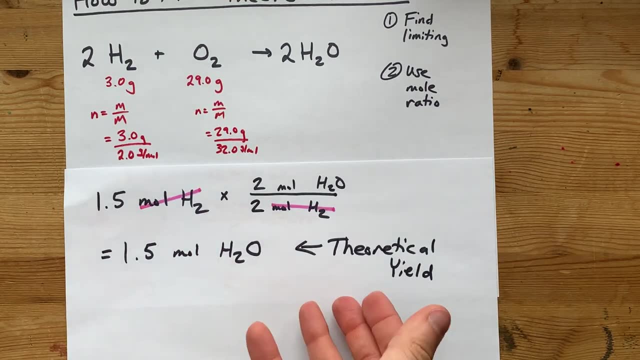 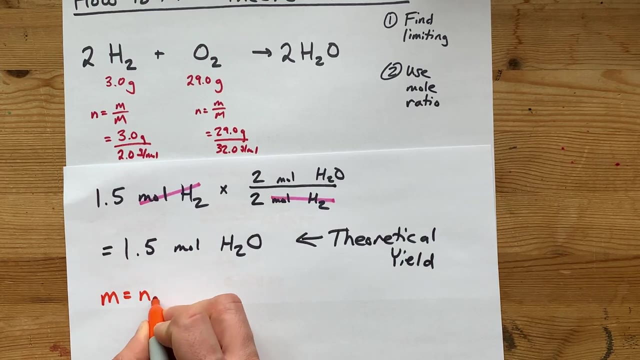 how much water, or rather your product, is made when your limiting reactant is used up totally. Now you may have been asked for grams of yield, like how many grams of it was made. That's a quick calculation as well. Mass is moles.